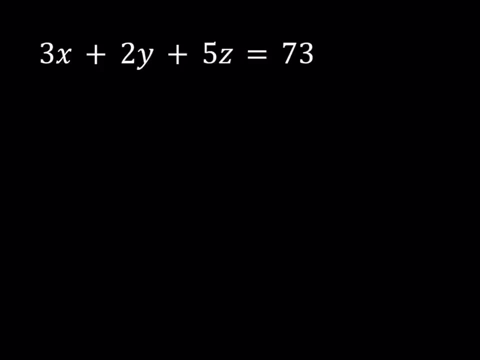 and it has three variables and we only have one equation. But we're going to be looking for integer solutions, All right, so we have 3x plus 2y plus 5z equals 73 and we're going to be looking. 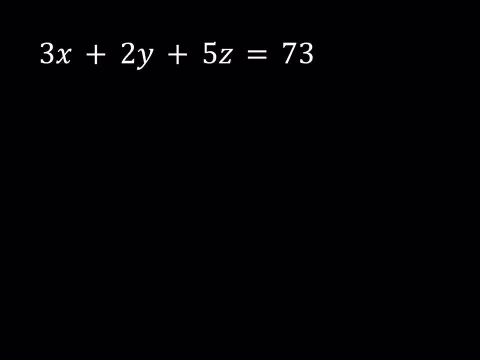 like I said earlier, integer solutions, not necessarily positive integer solutions. Okay, so how do we go about this? Well, for this problem we can easily use modular arithmetic, And I made a couple videos on modular arithmetic. I'll share the links as well. 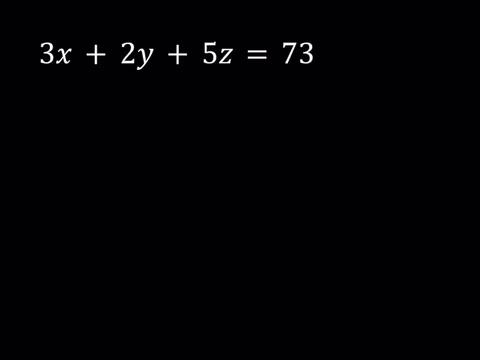 So now, what does that look like? First of all, looking at the coefficients 3,, 2, and 5, I think it would make sense if we used mod 2 and mod 3 here. So that's the plan. So what I'm going to do is: and what does that mean? Well, mod 2 means you're. 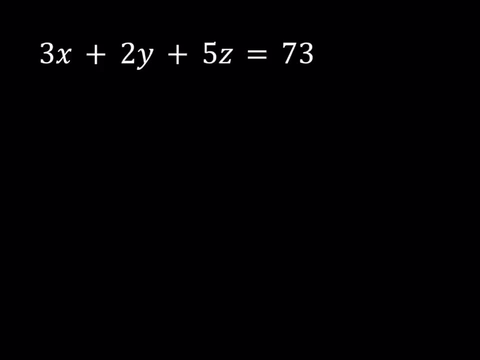 dividing everything by 2 and looking at the remainder. So it's kind of like the parity odd or even And mod 3 means you're dividing everything by 3 and looking at the remainders. Now what is that supposed to mean? Well, if this equation is true for a bunch of integers, 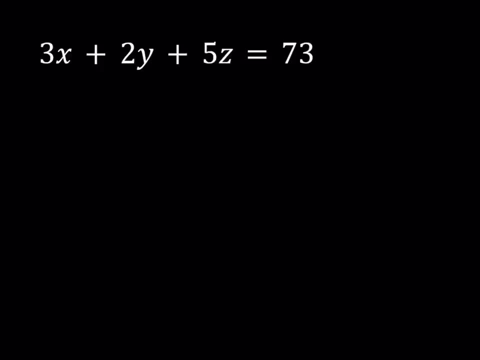 then when you check the remainders, it's also going to be true, right? When you divide everything by 2, if it's odd, it's going to be odd again, All right. so let's see what this gives us. 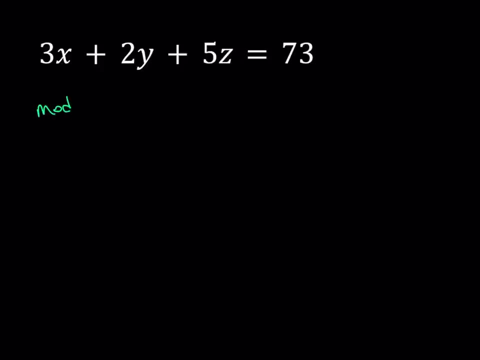 So first I'm going to use mod 2.. Mod 2 means everything will be reduced. For example, 3x 3, mod 2 is going to be 1, so it's just going to be x And y is going to disappear. That's also. 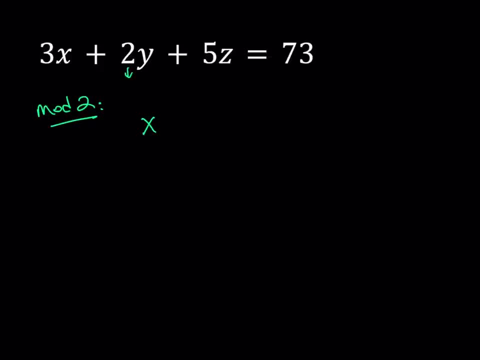 the good thing about it, We're not going to have y, because 2 is 0 mod 2.. That's why it becomes 0.. And 5 becomes 1.. Because if you think about, when I divide 5 by 2, what's the remainder? 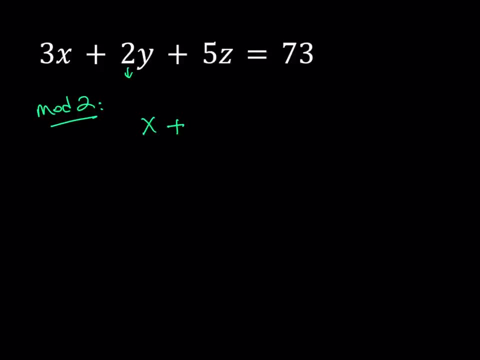 The remainder is 1.. By the way, mod 2 is also called binary because it's kind of like: well, not necessarily binary, but there's only two kinds of remainders in terms of that right: 0 or 1.. 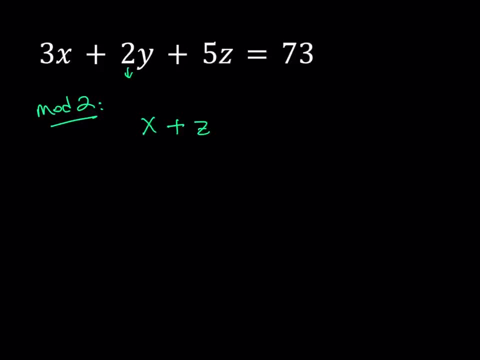 Okay, so 5z is just going to be z And 73, when you reduce it mod 2, it's just going to be 1, because it's an odd number. So we can write it as a congruent statement. x plus z is congruent to. 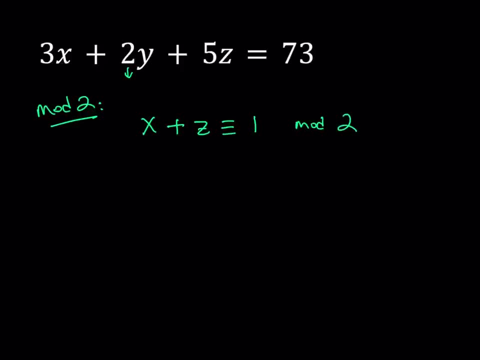 1 mod 2.. Of course, we have to state the mod here. Now what is that supposed to mean? It means that x plus z leaves the remainder of 1 when divided by 2.. So I can basically write it as x plus 2 is. 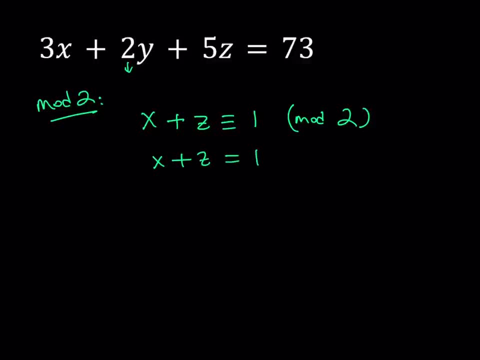 equal to x plus z, is equal to 1 plus 2k, where k is an integer. Okay, great. So that's one of my. obviously, I'm going to be using this later on. Let's go ahead and look at this equation. 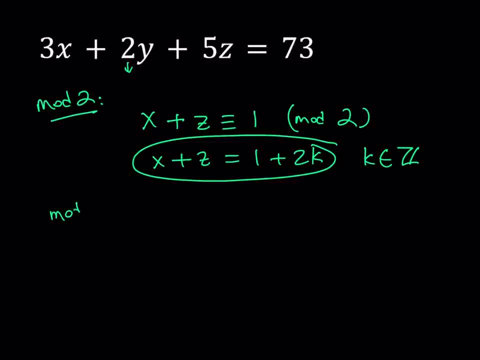 from another angle, which is mod 3.. The reason why I pick mod 2 and mod 3 is because of these coefficients. You might be wondering: why do I not use mod 5? You could? I mean that's there's. 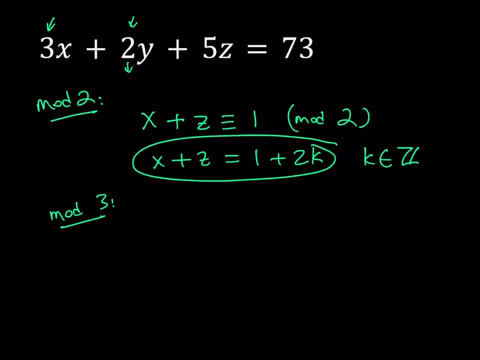 nothing wrong with that. So if I use mod 3, obviously x disappears, and then I get 2y, right 2y, and then 5z becomes 2z. 2z or not 2z? Well, it's not b right, I should have picked b. 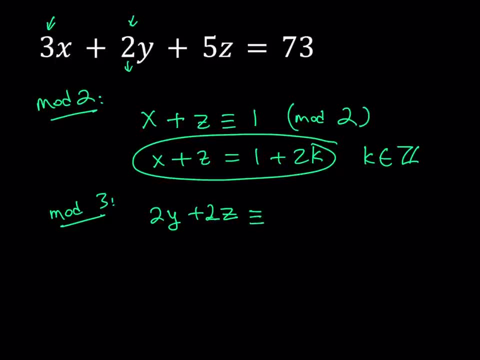 anyways, And this 73 is going to be mod 3, because 72 is divisible by 3.. That's going to be 1 mod 3, right? Well, I don't really like the 2s, because it's kind of like two evens. and now we're getting. 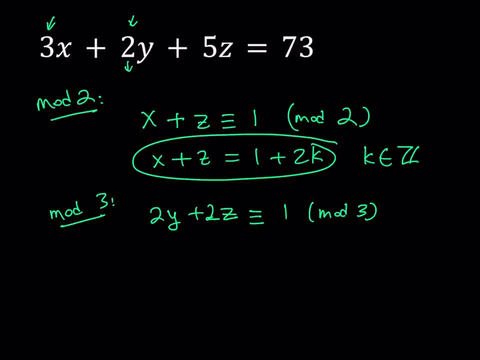 a 1.. Well, 1 mod 3 is not necessarily odd, of course, but I'd like to get rid of the 2, one of the 2s, So I can do the following: 2 is congruent to negative 1.. So I can just write this as a. 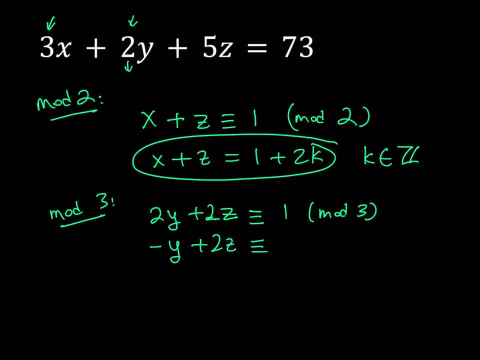 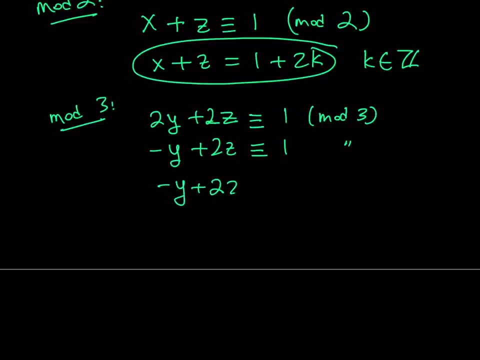 negative y, which is kind of cool, because having a coefficient of 1 is actually really nice. Mod 3,: right Now, I'd like to, of course, write it as an equality, not just congruence, So I can. 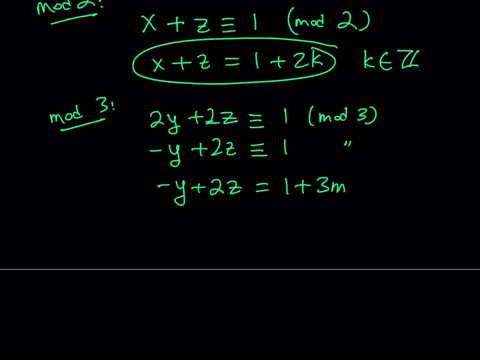 write it as 1 plus 3m, because anything that leaves a remainder of 1 when divided by 3 can be written as 1 plus 3m, where m is an integer, again, just like the other one, the k. Okay, of course. 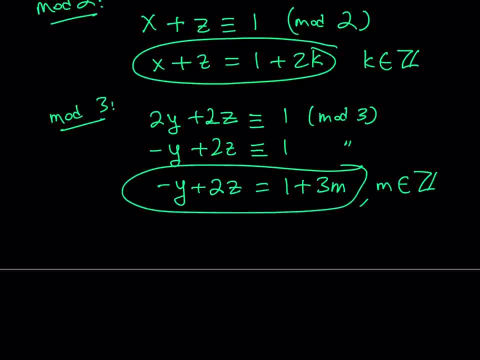 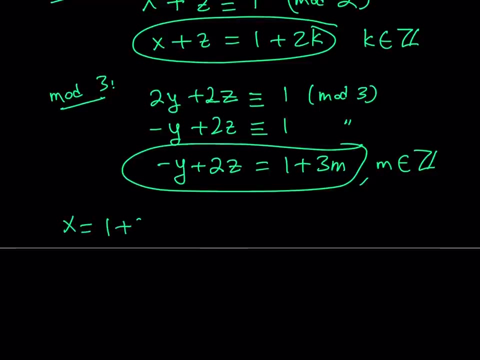 I'm going to be using this equation as well. So now let's see what happens. We have two equations for x and y. Well, we have z as well. So let's do the following: Let's isolate the x and y from these equations. So if I isolate x from the first equation, I get x equals 1 plus. 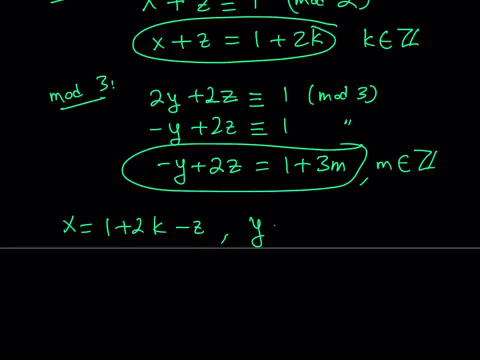 2k minus z And from the second equation I get, I have to put the y on the other side: 2z minus 1 minus 3m. So these are my two variables, in terms of the other variables, Of course, we introduced. 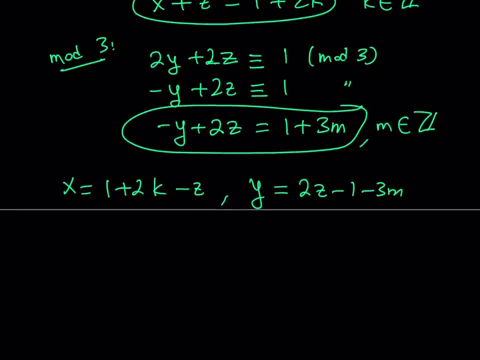 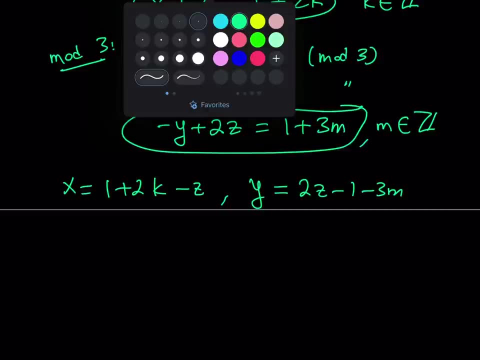 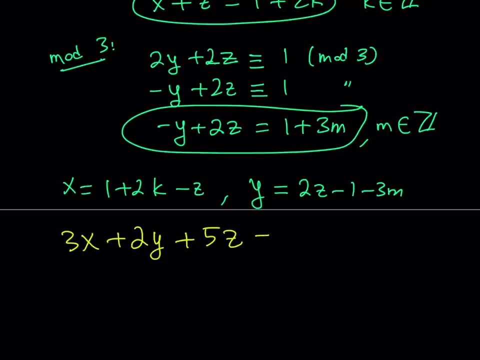 new variables, but that's okay, We're going to get rid of them. Now I have x and y in terms of z, and m and k, So let's go ahead and plug all these into the original equation. What was my original equation? It was: 3x plus 2y plus 5z is equal to 73.. Well, that would be perfect if I use ABC. 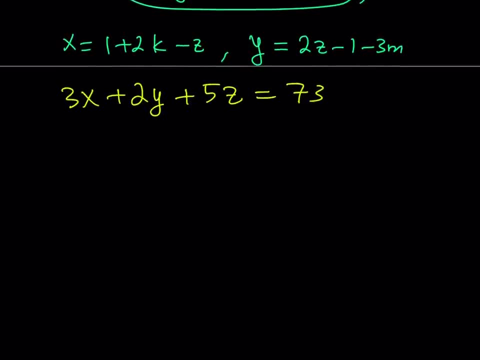 because I would have 2b. Anyways, that's okay. So now I'm going to substitute: Okay, x replaced with 1 plus 2k minus z, y replaced with 2z minus 1 minus 3m, And, of course, leave the z alone. 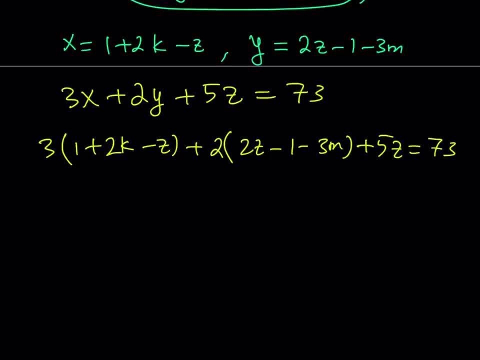 Now notice that everything is in terms of kz and m, And k and m are, by the way, just parameters that we use to express these variables, But at the end, we're going to use them to express all of them, all the x, y, z. 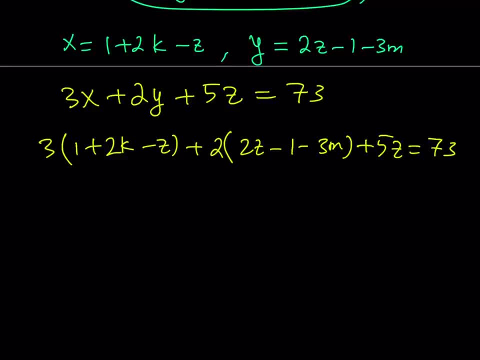 So now let's go ahead and simplify this a little bit, And that's going to look like: 3 plus 6k minus 3z plus 4z minus 2 minus 6m plus 5z is equal to 73.. And then let's go ahead and add these up. 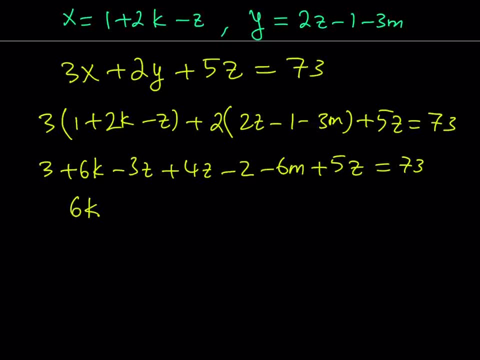 So from here I get 6k right and then minus 6m, And then z is going to give me. let's see what we get. This is 1z, and then plus 5z is going to be 6z, which is cool. That's really cool. And then I have the 3 minus 2,. 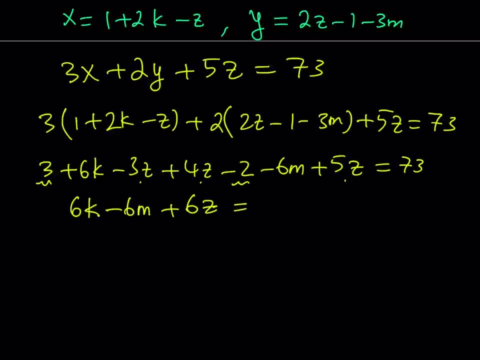 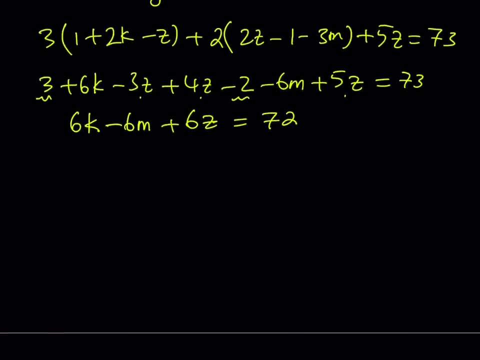 which is equal to 1.. If you subtract 1 from 73, you're going to get 72.. That's nice. Notice that everything divides out nicely. It's not always going to happen, but here it happened, and everything looks good. Everything is awesome. Okay, now divide by 6, you get something nicer. 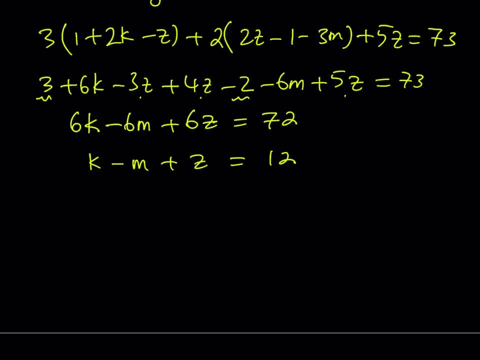 smaller numbers. Okay, great. So now what is that supposed to mean? Well, from here I can basically isolate z right, So I can write z as what 12 minus k plus m. So this allows me to express z in terms of k and. 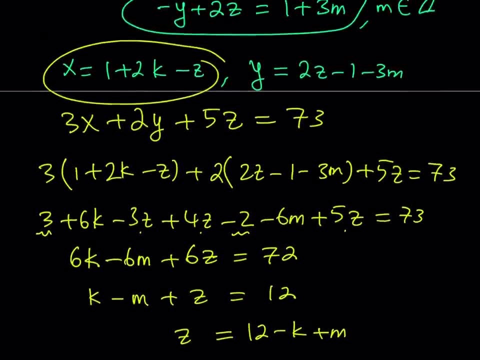 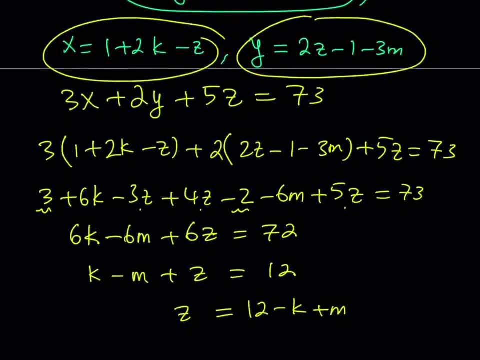 m And notice that we had x and y in terms of z and m, z and k before. So now, how do you put these all together, right? Well, here's the thing. Now I got an expression for z, So what? I'm going to do is: I'm going to put this all together And I'm going to write this expression for z. So what I'm going to do is I'm going to put this expression for z. So what I'm going to do is: 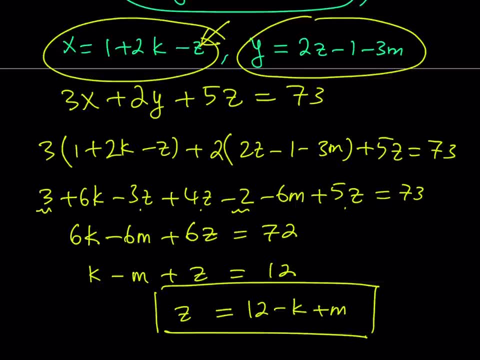 I'm going to do is note that we have z here and here. I'm going to replace those z's with this one. Make sense? Great, So let's go ahead and do that. I have x equals. I have x equals 1 plus 2k. 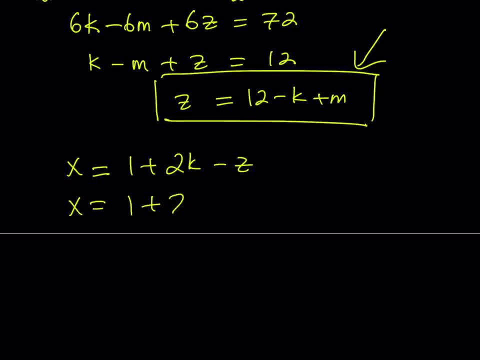 minus z, And let's go ahead and replace z with what it is here: minus. let's write that in parentheses and then simplify that. Let's go ahead and simplify this expression. Let's see what happens. So if you simplify, you get 1 minus 12, that's a negative 1, negative 11, I mean 2k. 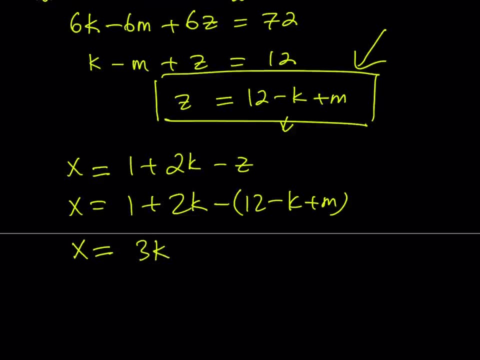 plus k is going to be 3k. right, That's going to give me 3k minus m, because m is positive, but we're going to negate it. 1 minus 12 is going to be negative 11.. Okay, so that's my x value, and 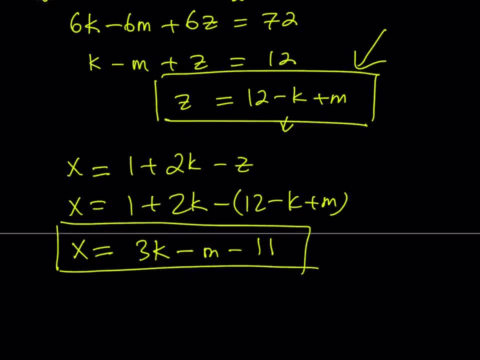 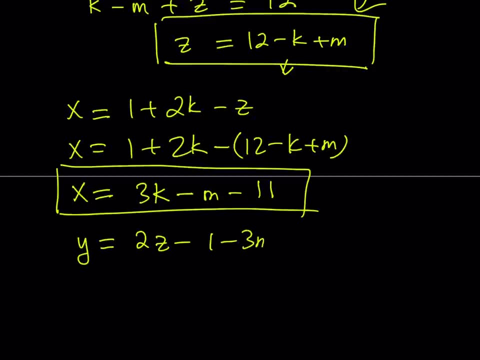 I should frame that because that'll be important. Let's do the same thing for y. What is y? Well, y is equal to, if you remember, it is equal to 2z minus 1 minus 3m. And now I'm going to replace z with what it is, and z was this expression, Remember here. 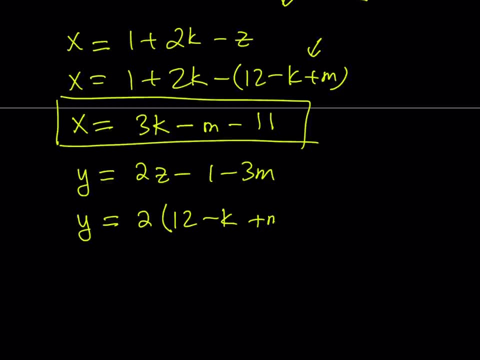 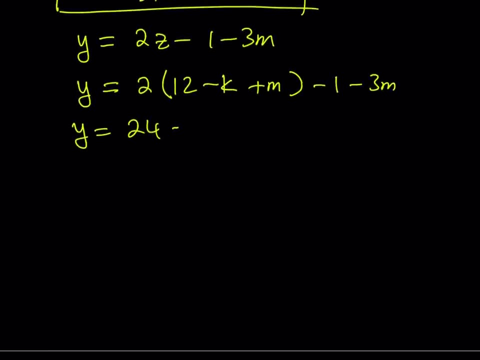 2 times the quantity, 12 minus k plus m, and then minus 1 minus 3m. Let's simplify this: 24 minus 2k plus 2m minus 1 minus 3m, And from here, From here, y becomes what Let's see. 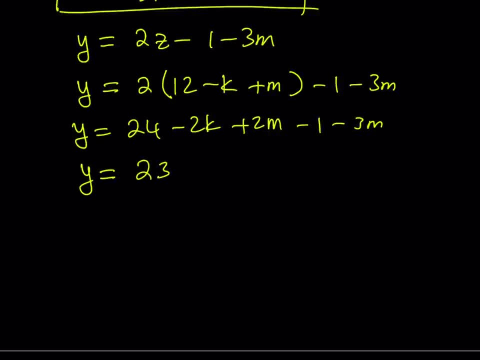 I'm going to get 24 minus 1, which is equal to 23,, and then minus 2k, 2m minus 3m is equal to negative m. so I'm going to be getting 23 minus 2k plus m for y. 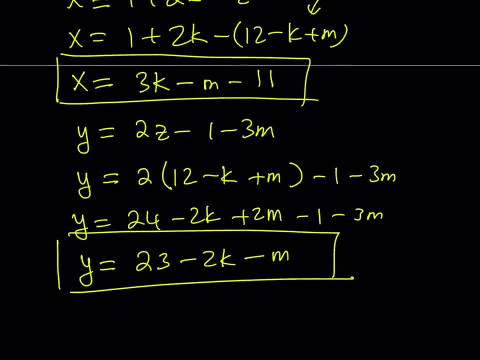 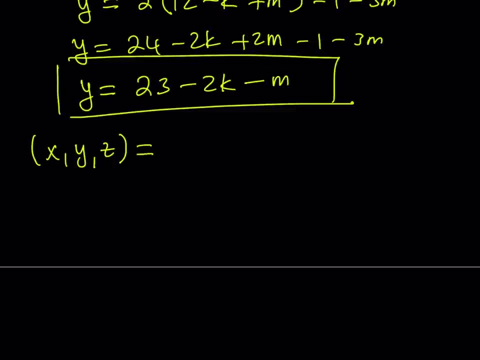 And what happens here is we got the x and we got the y and we already had the z in terms of everything. Let's put it all together and I'm going to show you a couple examples what this means. So x, y, z has an order. triple can basically be written as now: 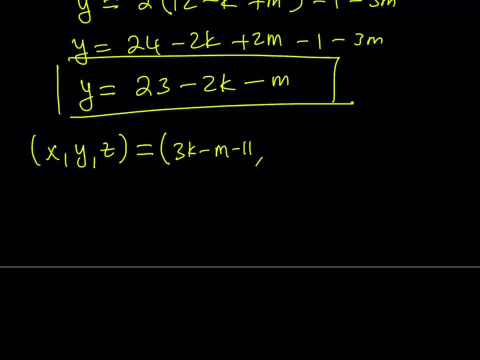 3k minus m minus 11, comma 23. minus 2k minus m- comma 12. minus k plus m. That basically gives us all the solutions, but let's go ahead and look at some specific ones. For example, what if k and m are both 0?? 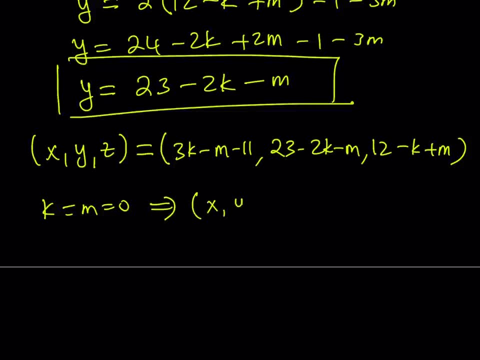 From here we kind of get a simpler solution, because it's easy to substitute right, k and m, basically forget about them And you're going to get negative, 11, right, And then you're going to get 23 and 12.. 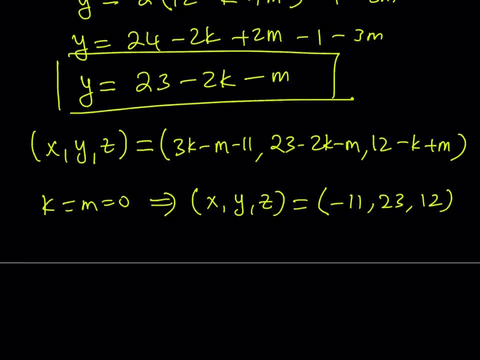 So you can satisfy like. you can go ahead and plug these into the original equation. you're going to notice that they satisfy the original one. And let's take a look at another case: k equals 1, m equals 0.. 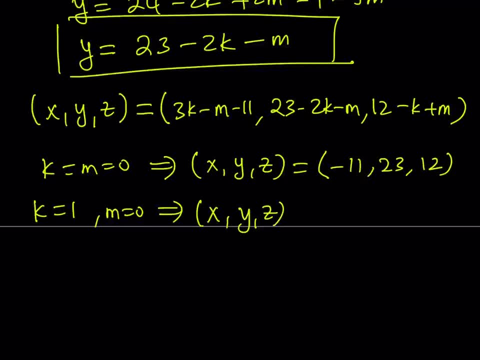 It's going to give you another order, triple x, y, z- and that's going to look like negative: 8,, 21, and 11. And then, finally, let's just do something different so that we can get a nicer solution. 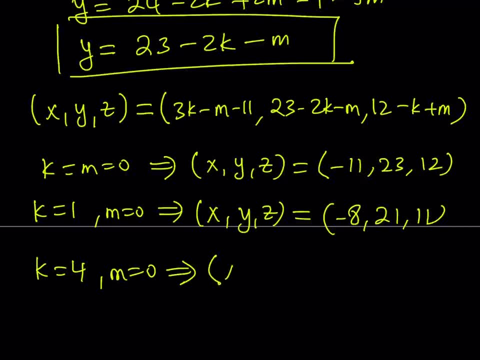 I'll tell you why it's nicer If you do: k equals 5.. 4 and m equals 0. And notice that I'm always trying to stick to 0. Sometimes you don't have to do it, but I'm just going to show you something here. 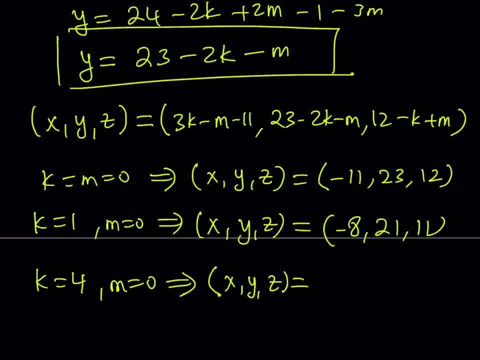 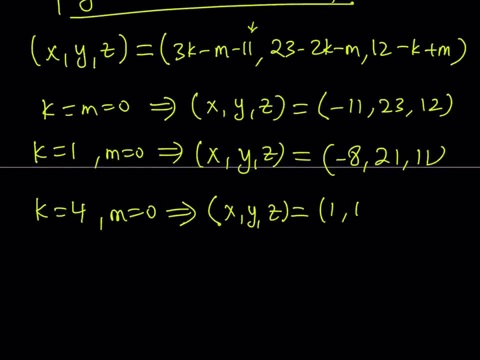 The reason why I pick a large k here is because I want to get rid of the negativity of the 11 here so that I can get a positive answer. That's the goal, And we get 1,, 15,, 8. And this is going to be my positive solution. okay. 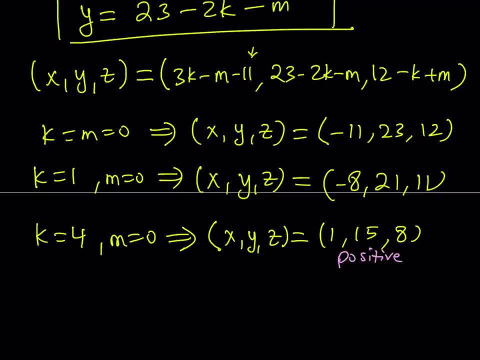 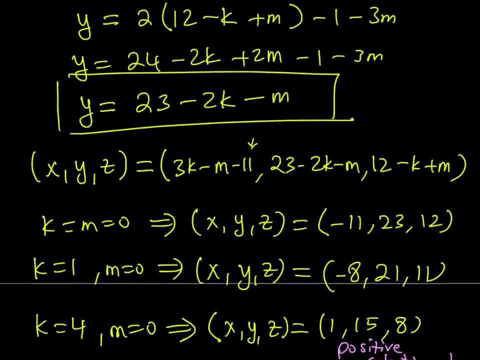 So this is going to be the positive case, And are there any other positive solutions? Check it out, Find out And just let me know, But this is the one that I found. So, basically, our solution consists of this: order triple, where k and m are both integers. 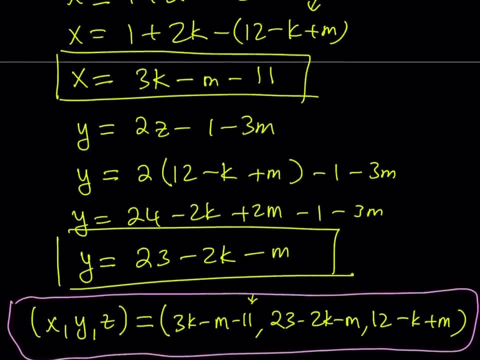 And basically you can express the solution as like a parametric solution here, which means that you can run through all the values of k and m as long as they're integers, and you can get infinitely many solutions to this linear Diophantine equation. 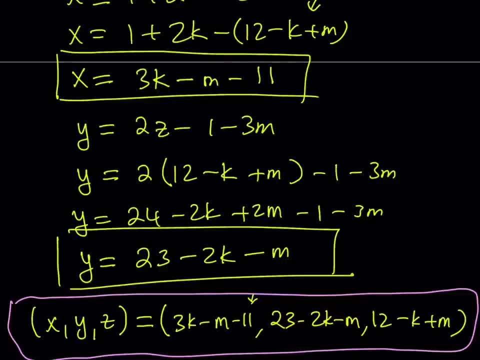 Well, this brings us to the end of this video. I hope you enjoyed it. Please let me know. Don't forget to comment, like and subscribe. I'll see you tomorrow with another video. Until then, be safe, take care and bye-bye.